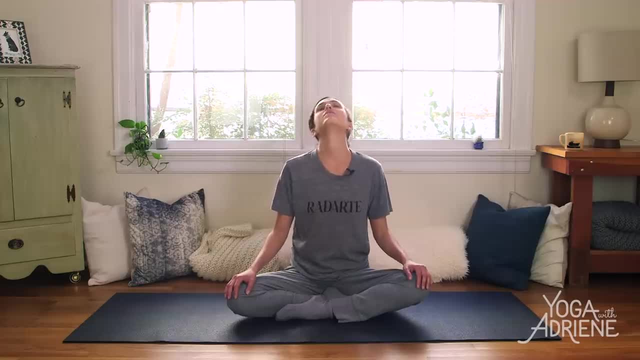 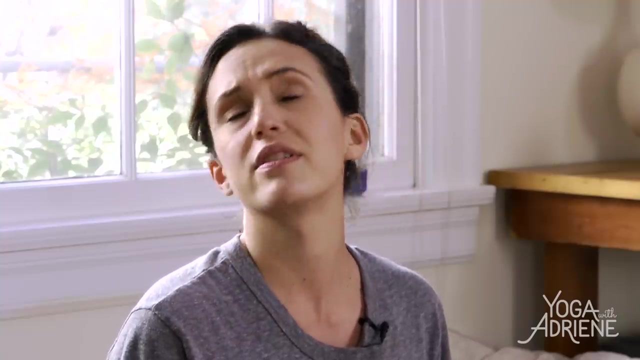 We're going to take a few deep breaths And then reverse your circle, Move in the opposite direction, Keep the shoulders relaxed here and enjoy this beautiful time that you have carved out for yourself. Maybe you feel like, oh, I don't even have the time, but relish in this. 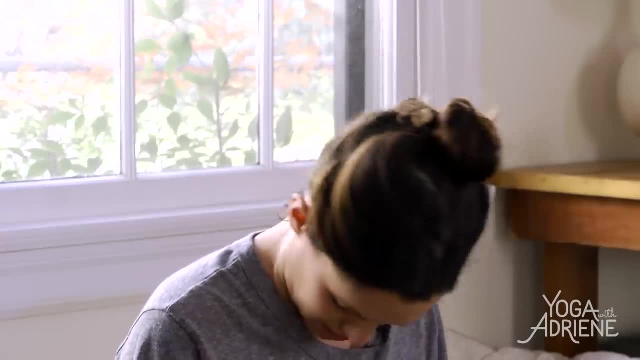 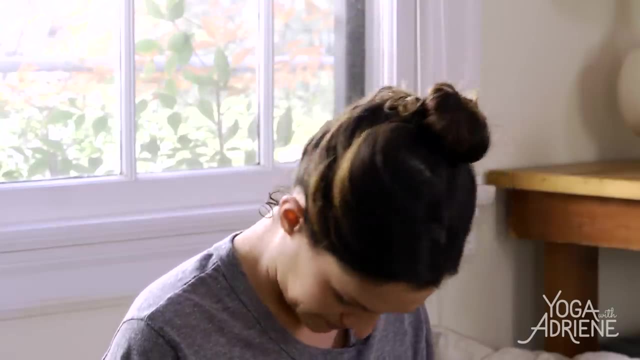 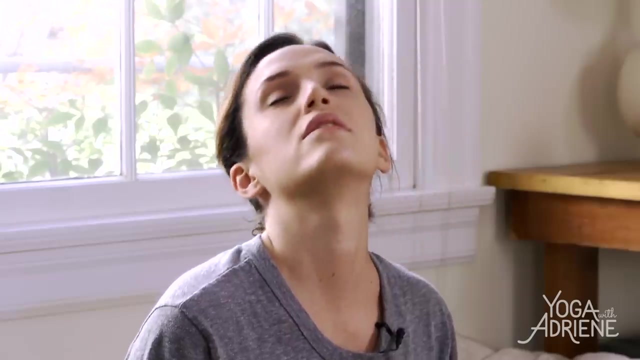 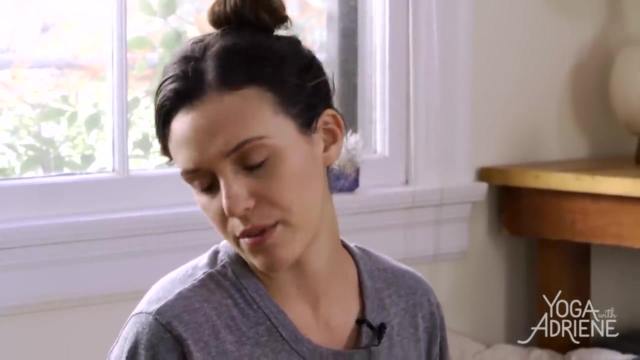 awesome bedtime practice, Knowing you will benefit from it. Connecting the brain and the body, mind intelligence and the body: intelligence. Winding down for the day. Reverse your circle one more time. If you find any catches here, you might rock back and forth there. 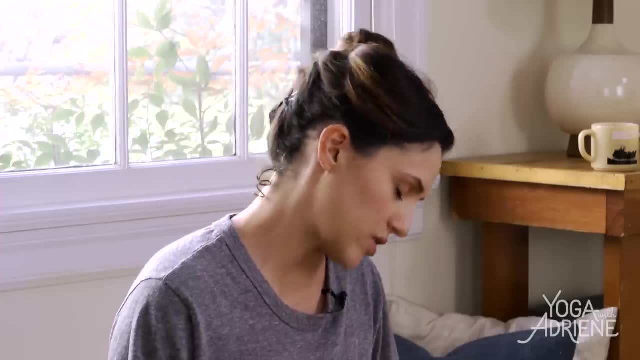 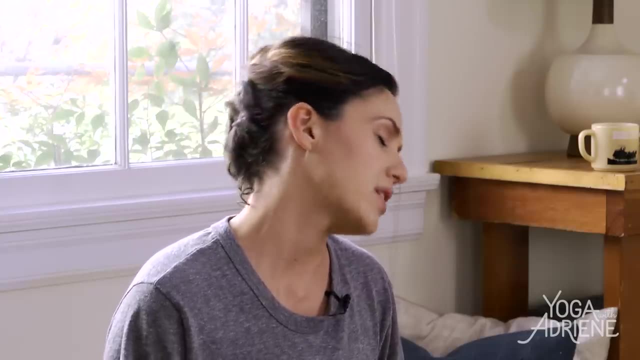 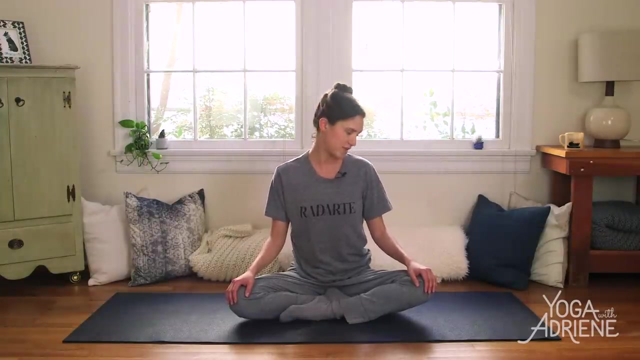 Just finding a little movement here that feels good. You might feel a little weird doing it, but if you just close your eyes and surrender, find what feels good. And then one last breath here. Find what feels good, Letting go of the stress and the tension that perhaps is built up over the course of the 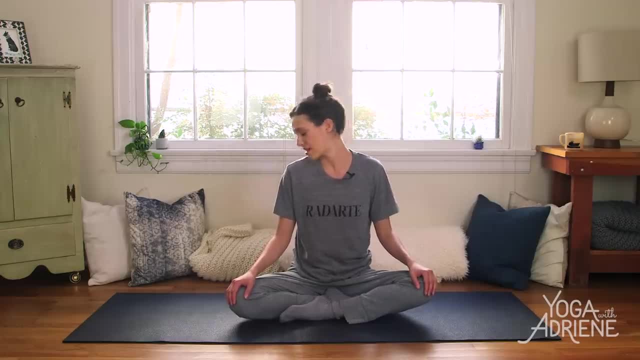 day, And then we'll bring the head back to center. Draw the palms together at the heart, Take a deep breath in On the exhale, bow your head, And then we'll bring the head back to center. Draw the palms together at the heart. 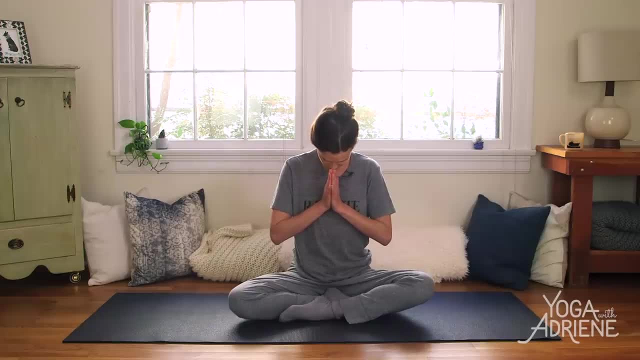 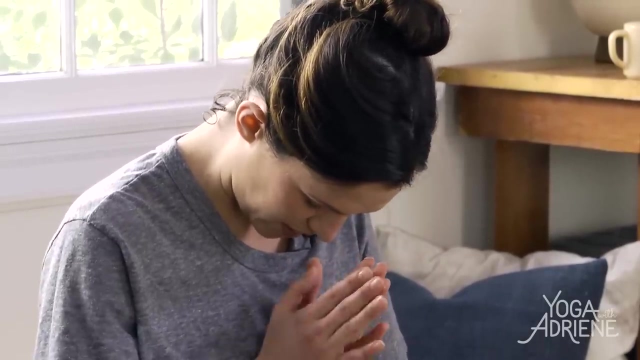 head, to your hands, to your heart. now actively draw the shoulder blades together here, breathe into the back of the neck, close your eyes, feel the sensations of the palms kissing together at the heart and prayer one more breath. here you might imagine a little trapdoor opening out through the crown of the 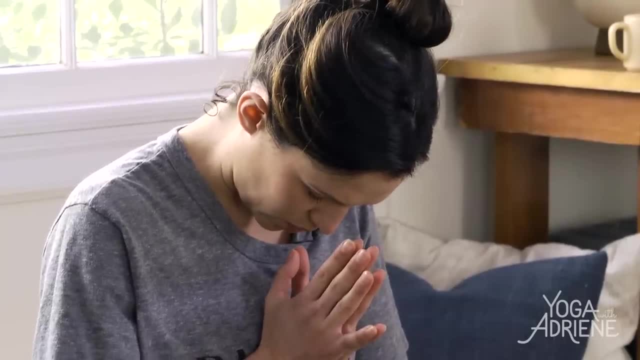 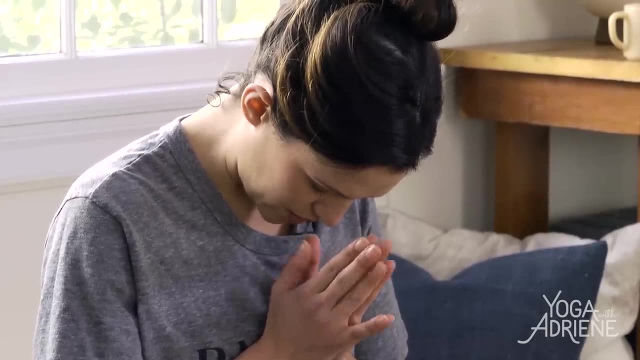 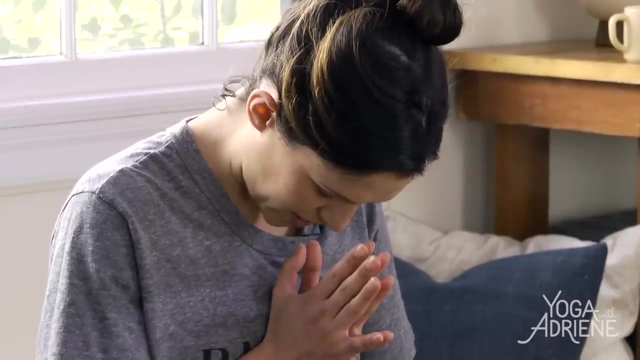 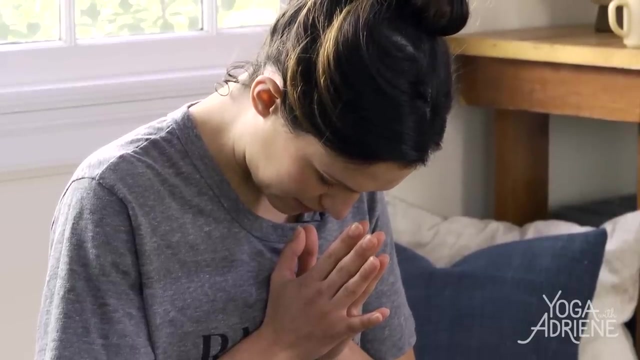 head and again, any stress you've been carrying, any tension, any worry, any burden of the day or even anything in anticipation of the future of tomorrow. just go ahead and let it spill out, trickle out, telling the mind, the body, the heart that we are winding down for the day, preparing for much-needed rest. 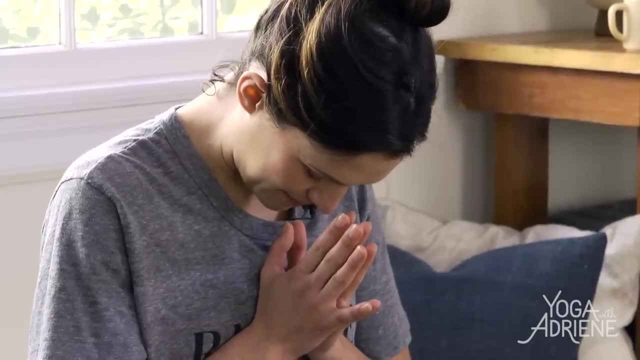 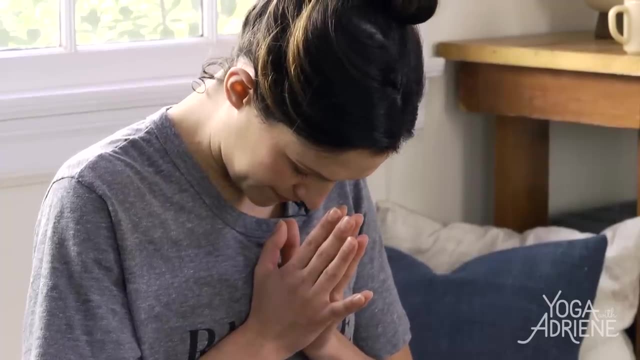 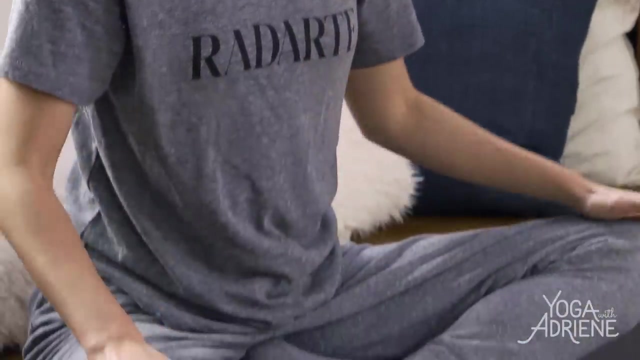 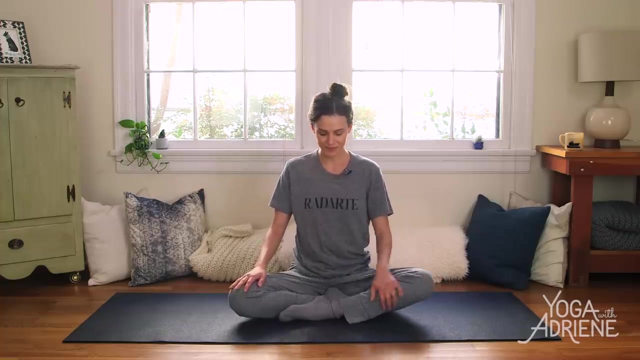 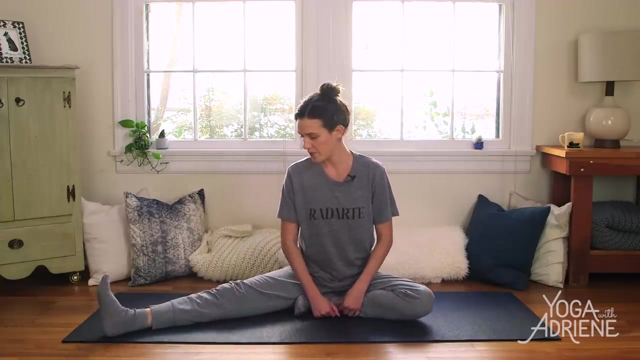 balancing the equilibrium, finding peace from within your inner self with a breath of breath in, big breath, in big breath out. release the fingertips down to the legs- nice- and slowly roll up through the head of the neck- awesome. so we're going to draw the left heel in towards the center. 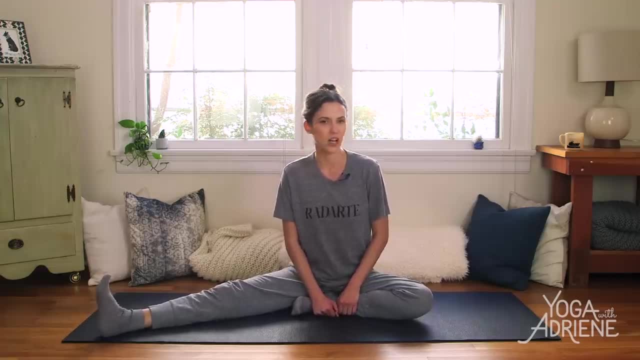 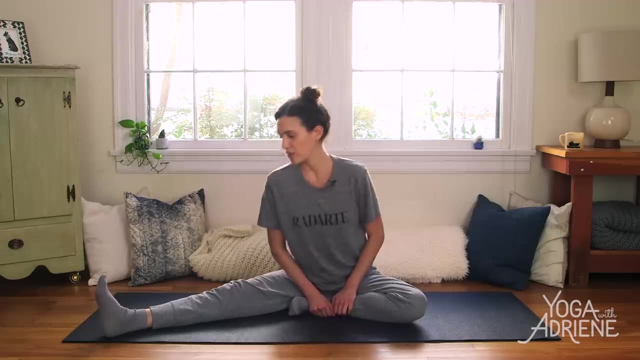 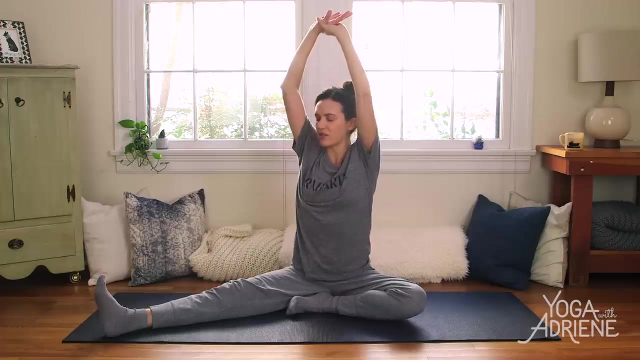 and extend the right leg out long today, Point and flex, point and flex, And then, when you're ready, we're gonna reach the arms, just nice and soft and slow all the way up. Take a nice big stretch here, Lengthening, uncrumpling, lifting up on all four sides of. 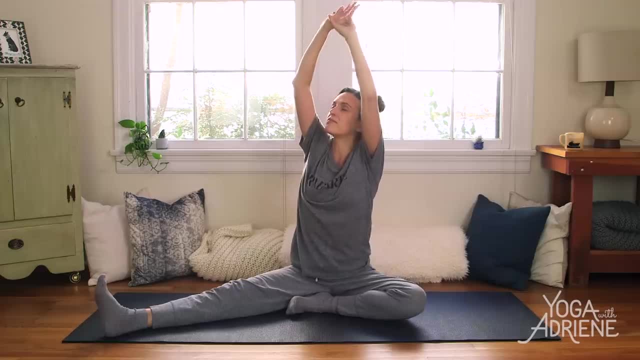 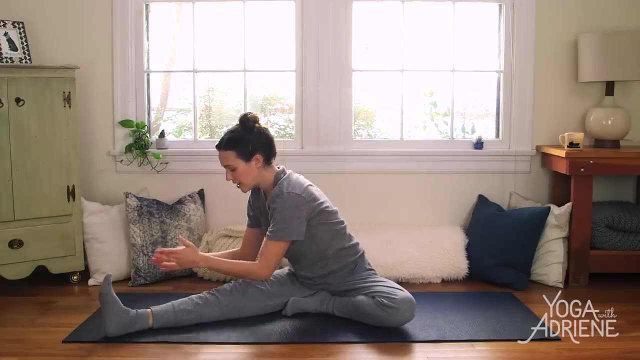 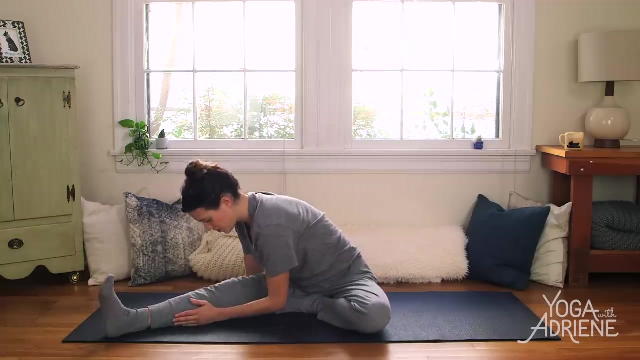 the torso, so the side body, the front body, the back body lifts And then exhale softly, release, Begin to turn towards your right foot and find a place where you can bow the head, So it might be a kind of classic Janu Sirsasana head to knee pose. 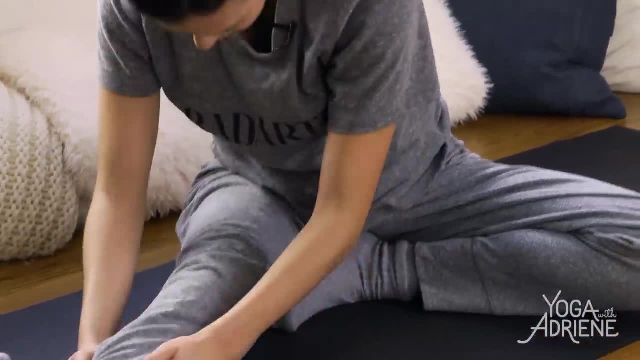 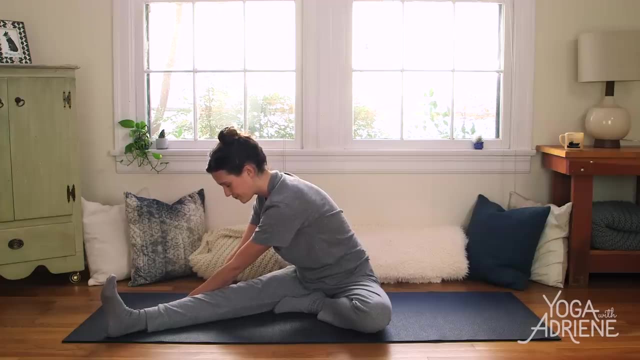 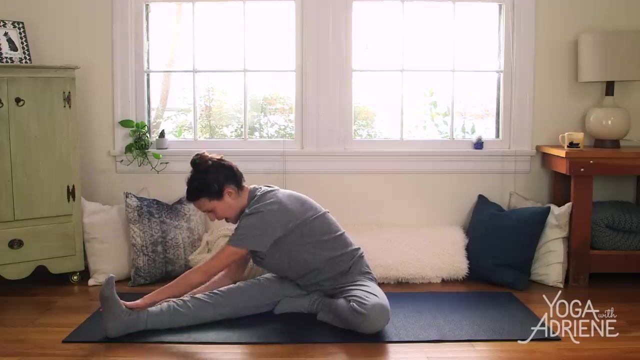 Janu Sirsasana. Or you might keep it nice and chill, just kind of resting here, maybe reaching to the outer edge of your right shin. Your body's gonna tell you what feels awesome. So if it's lower back body, you're here. If it's the leg, if you need a little. 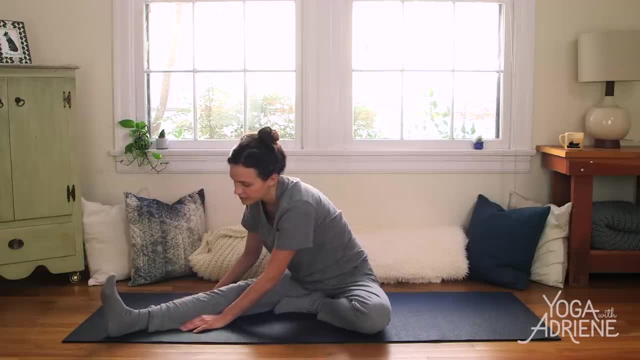 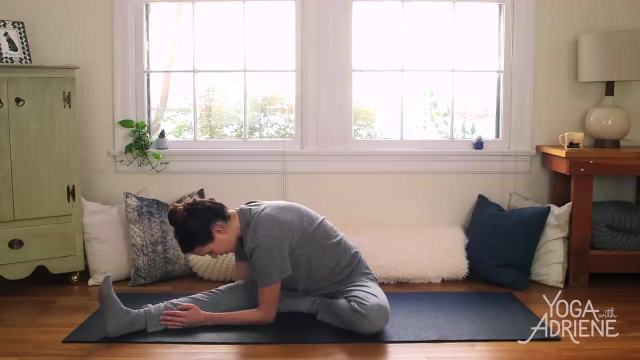 twist Everyone. see if you can keep the right foot bright. So, even though we're working softly and mindfully, see if you can keep a little energy in that right foot. Then come to a place that feels good and allow the eyelids to soften or close. 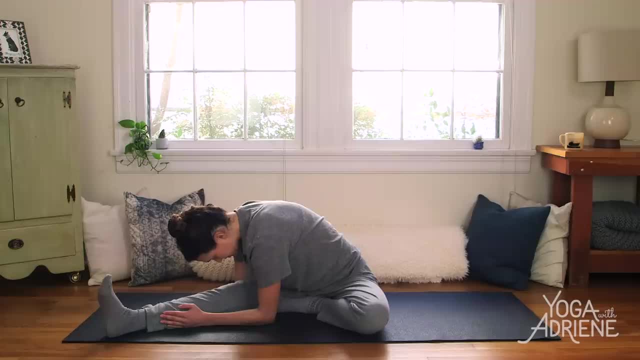 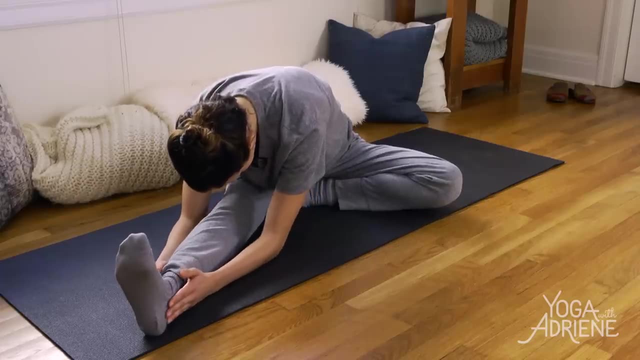 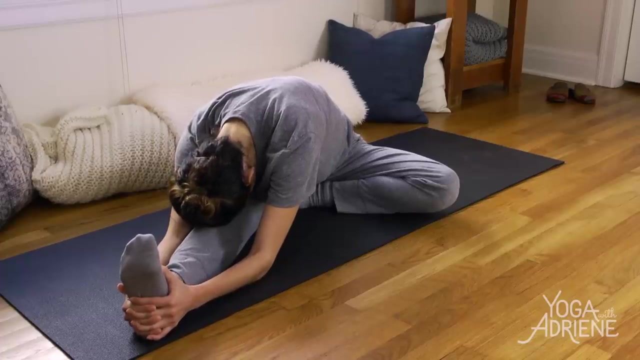 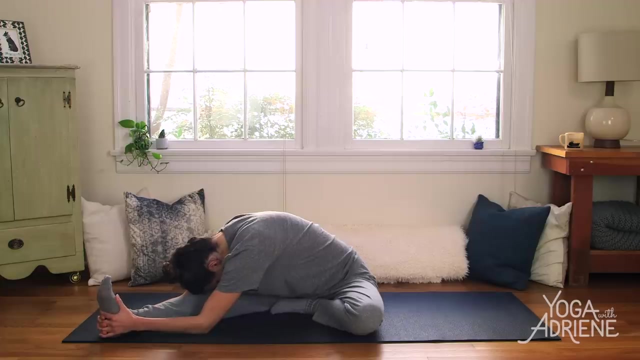 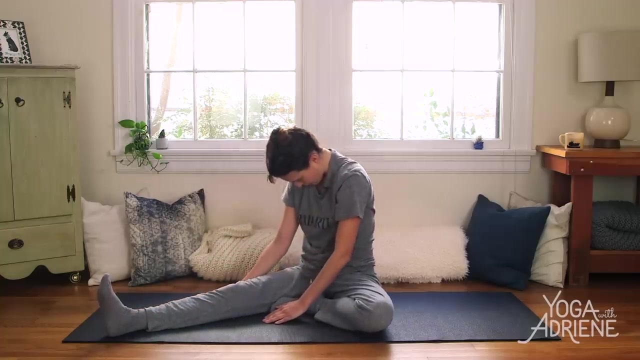 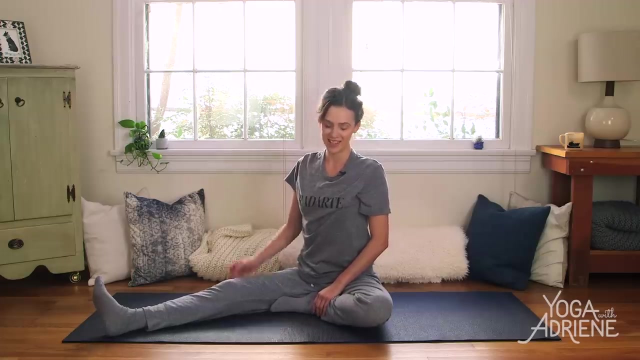 Make your inhale long. Exhale even longer And then exhale. Listen to the sound of your breath here And then slowly release wherever you are, tuck the chin into the chest, Roll up through the spine. So much love here. as we roll up through the spine, Inhale, lift the chin and chest. 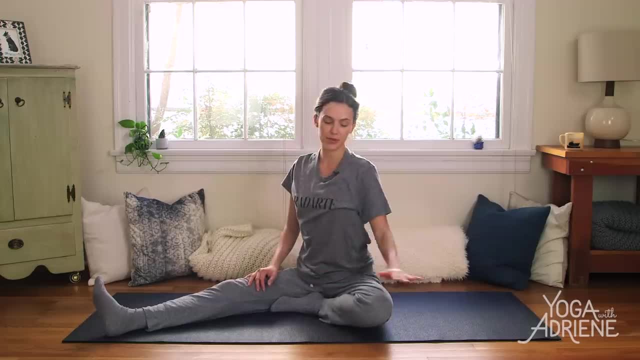 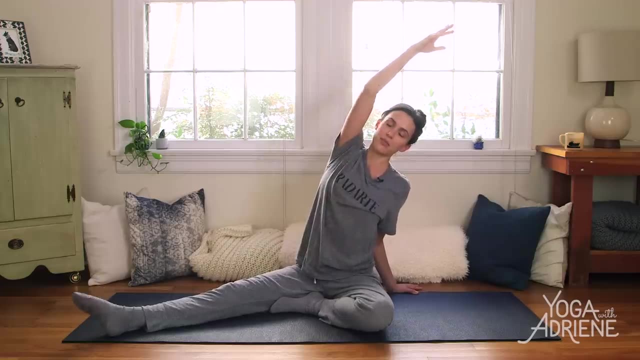 And then on an exhale, just a little counter pose. we're gonna take the left palm behind or left fingertips and inhale. sweep the right arm all the way up and overhead. This time point your right toes, breathe in here. 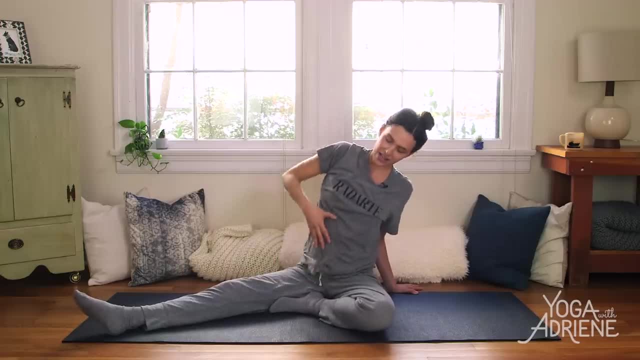 Don't really worry about the perfect shape, but your body will tell you: ah, yes, opening. So we just fold it. and now we're gonna open, Inhale in and exhale back to center Great, draw the right heel in, left leg out. 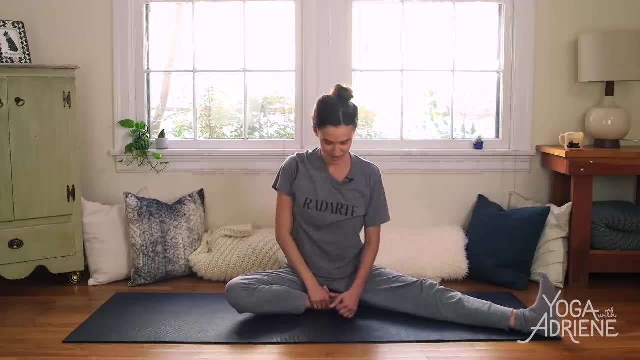 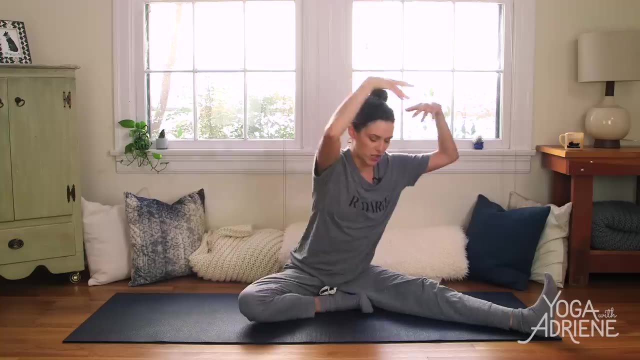 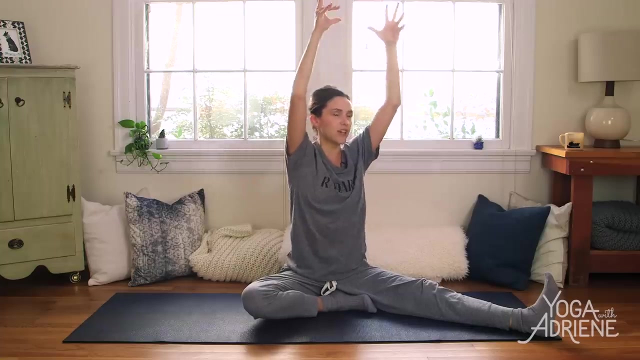 Take a second to get set up here And then, when you're ready, inhale, reach for the sky. nice and slow, Experiencing the body stretching, slowing everything down. Inhale, lift through all four sides of the torso. 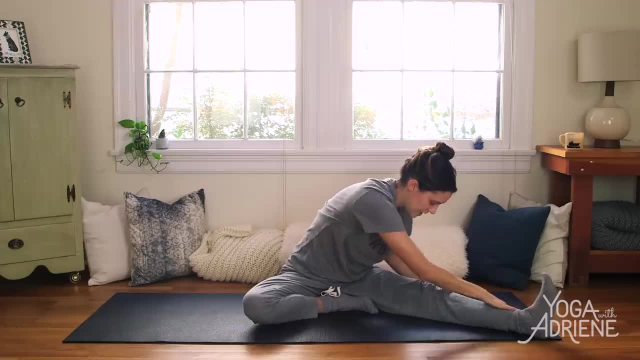 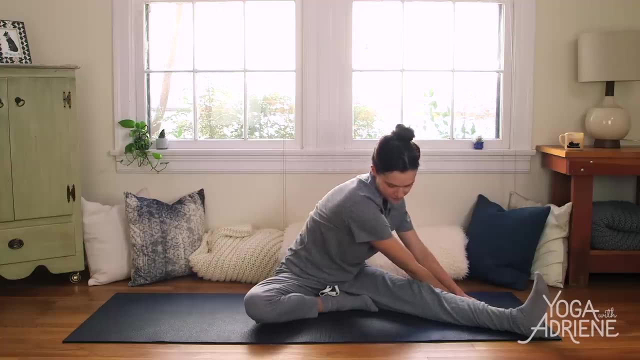 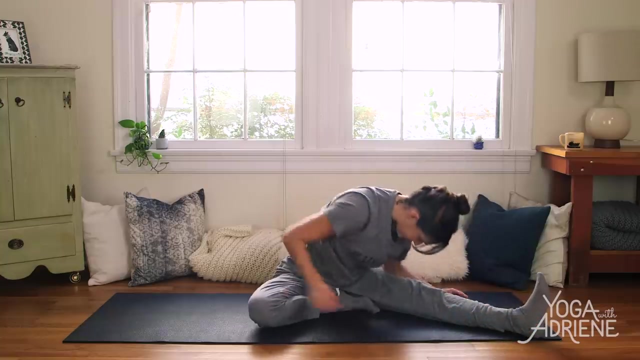 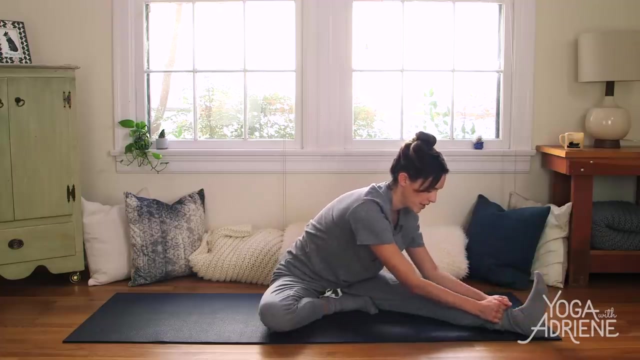 And exhale, rain it down. So each side is different. here You might come to the outer edge of the left shin. You might come to Head to Knee Pose, Maybe interlacing around the foot or holding on to your pant leg. 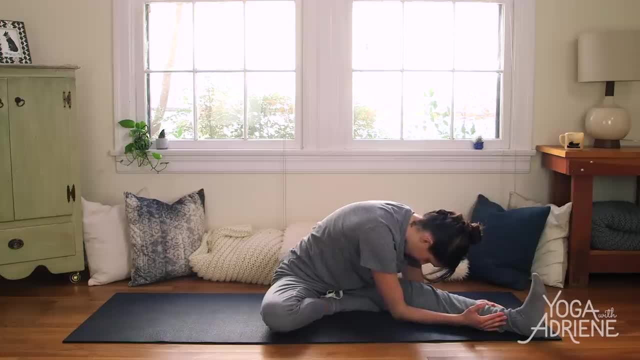 Finding the breath again here, softening through the forehead, closing the eyes or finding a soft gaze, Allowing again the day thus far to melt away in the anticipation of tomorrow, to hold being present with your body, in your breath. This is an act of self-love here. 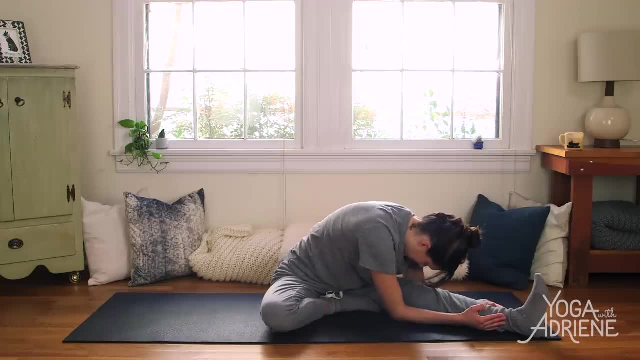 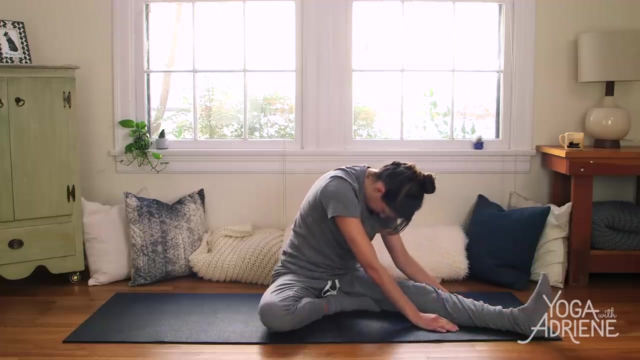 And super great for the body. One more breath here, wherever you are, enjoy Inhale, exhale, Inhale, exhale. And then slow wanna hold, slide back, Slowly release, Tuck the chin into the chest. 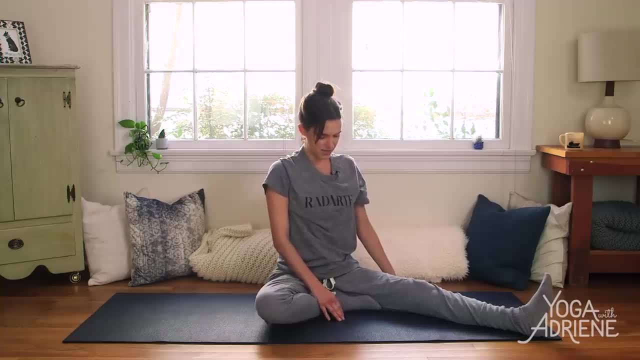 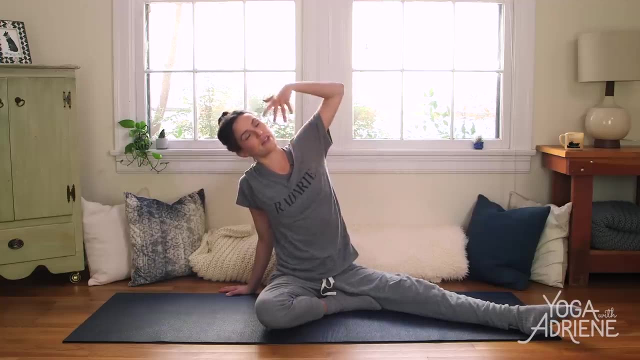 Stacking head over heart, heart over pelvis, Beautiful. And then releasing the right palm back, pointing through the left toes and inhale, Reach left fingertips up high. Big breath in, Big breath out Brings you back to center. 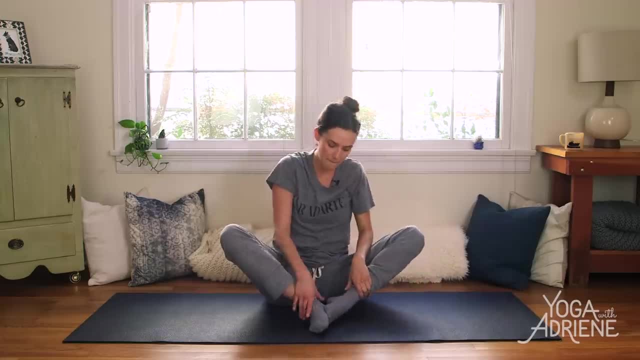 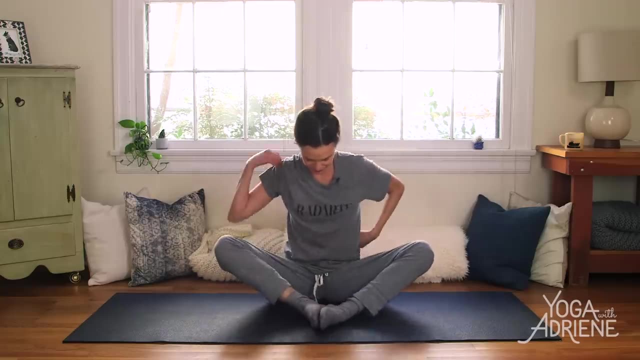 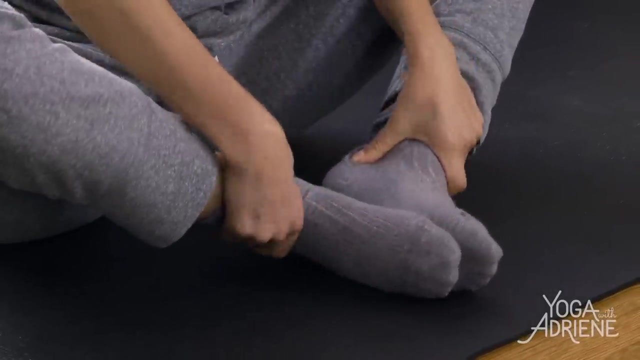 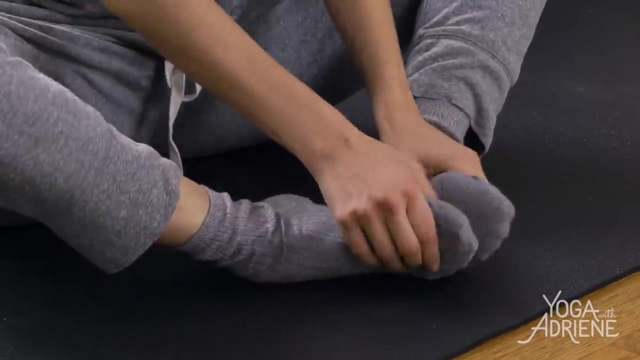 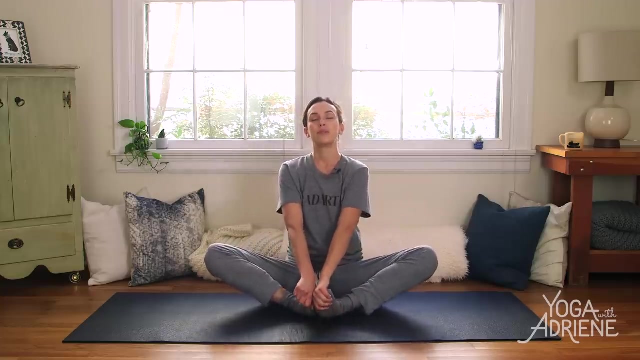 Awesome work. Soles of the feet come together here, So take a second to give yourself a little foot massage. Thumbs coming to the ankles or the arches, The heels And the base of the foot, the toes Keep breathing here. 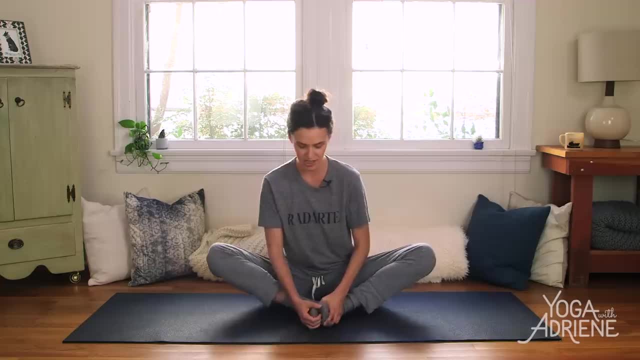 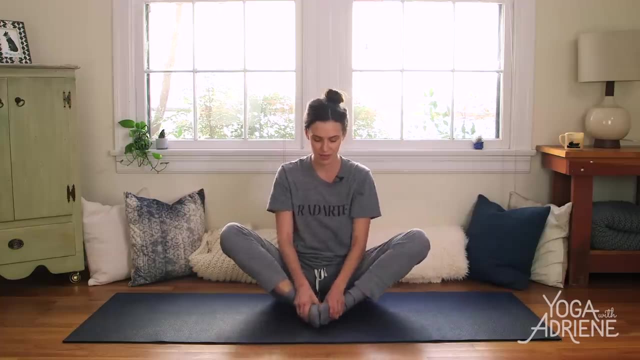 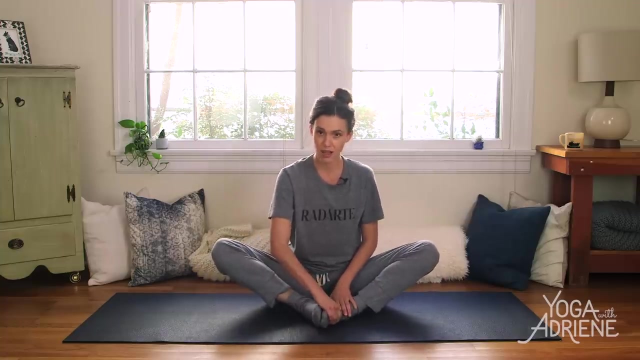 The more you practice this video, you can freestyle here, finding extension through the foot, Maybe even lifting both legs. But if this is your first time, just keep it to a nice, soft, gentle massage. Maybe you start to bring oils into the mix. 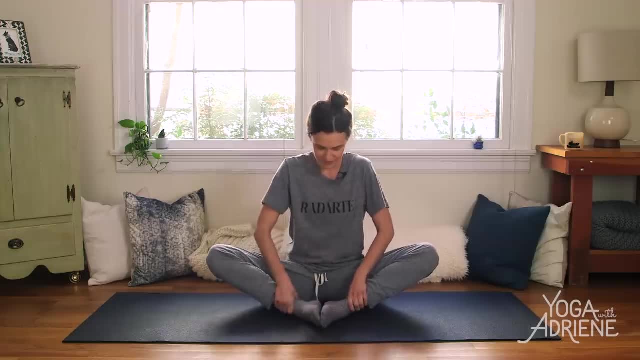 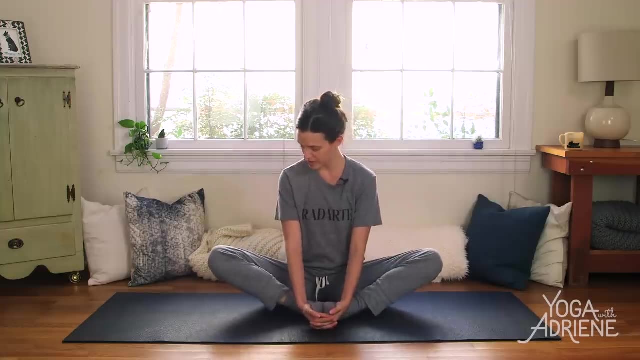 Little lavender oil in the feet, Mmm. And then we'll interlace the fingertips, Bring them to the toes. Bring them to the toes and draw the tops of the thighs down As you inhale. lift the heart As you exhale. drop the chin to the chest. 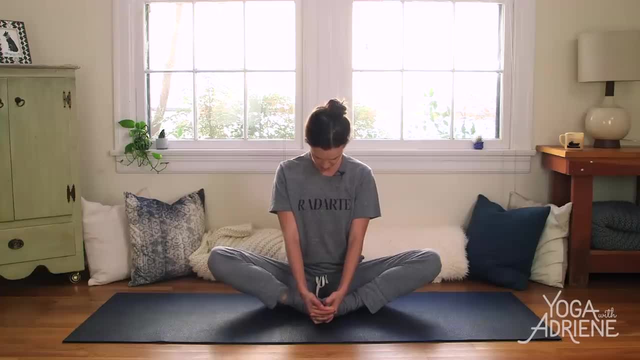 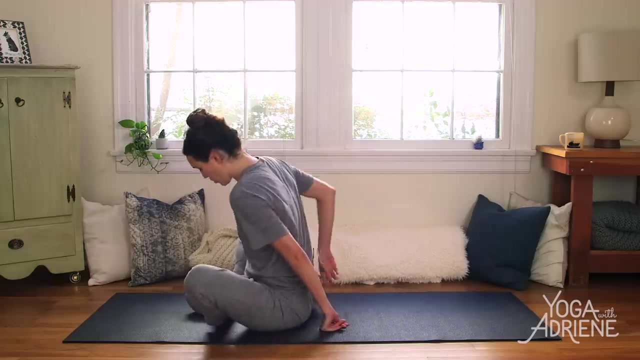 Close your eyes, breathe here, Grounding down through the tops of the thighs. Inhale in, lift your chin, Exhale, swim the fingertips around. So fingertips are gonna come behind you now And we're gonna keep the soles of the feet where they are. 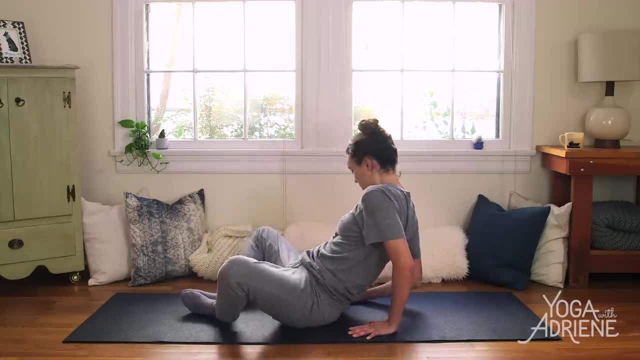 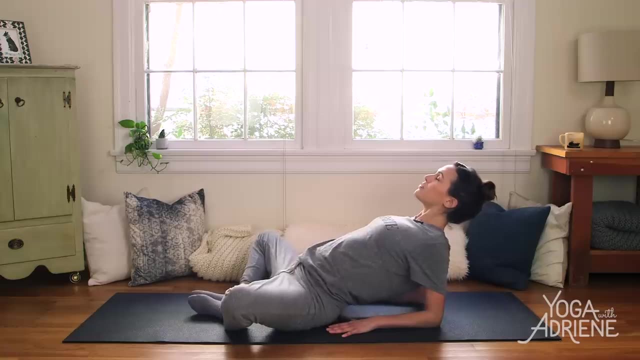 As we walk ourself back, This time to the elbows, Keep the legs as they are in Baddha Konasana. Inhale in open the chest, Breathe, breathe, breathe, Exhale. continue the journey down. 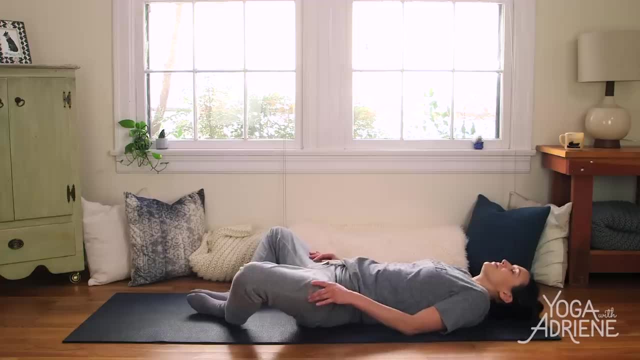 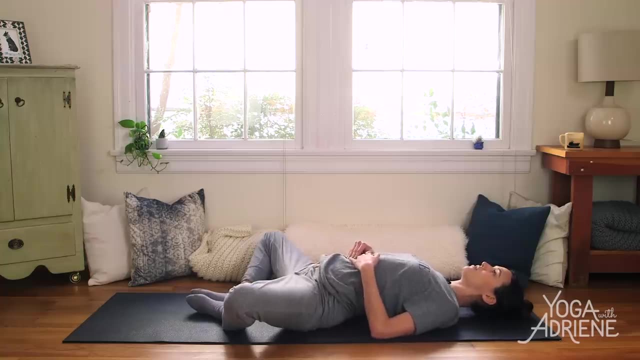 All the way to the back. Oh yeah, Now we're talking. shoulder blades Shimmy underneath the heart space here. So crawl the shoulder blades underneath you, Hands come to the belly And the legs grow heavy If you're feeling any pressure at all. 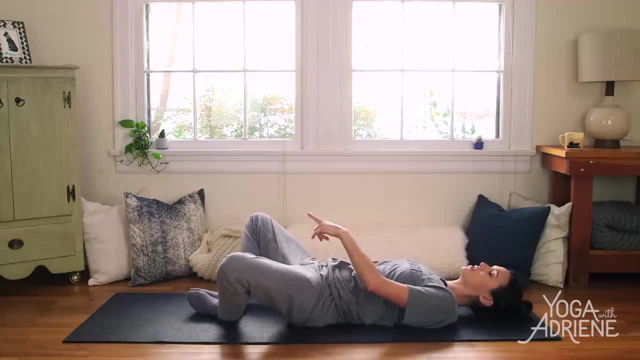 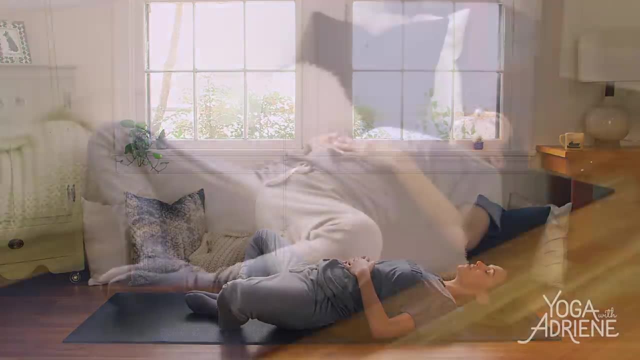 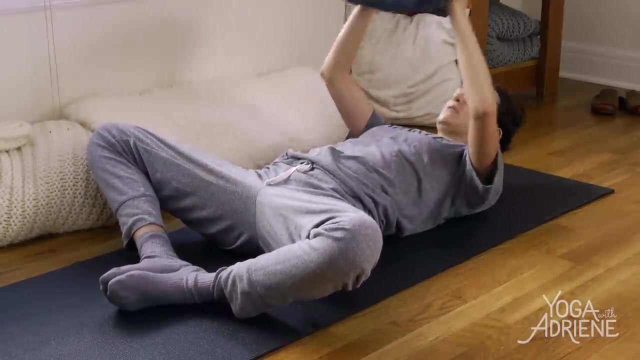 in the lower back. my loves, lift the tail, draw it down towards your heels And then release back into this restorative posture. So this would be a great time to maybe pull a blanket or a pillow- I'll choose you- Underneath the head or the neck. 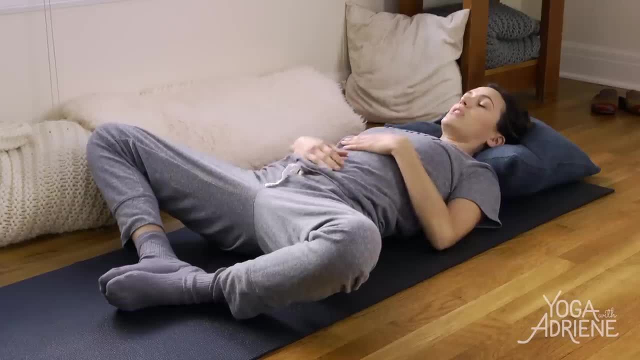 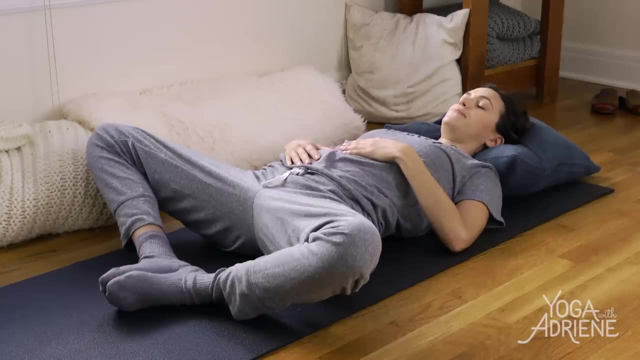 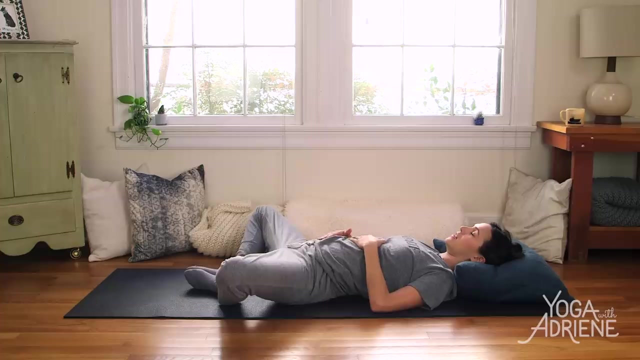 Oh yeah. And then actually I want to keep the hands on the belly because I'd like for us to breathe into the belly here. So once you get situated, close your eyes And just with the sound of my voice here we're gonna inhale in big. 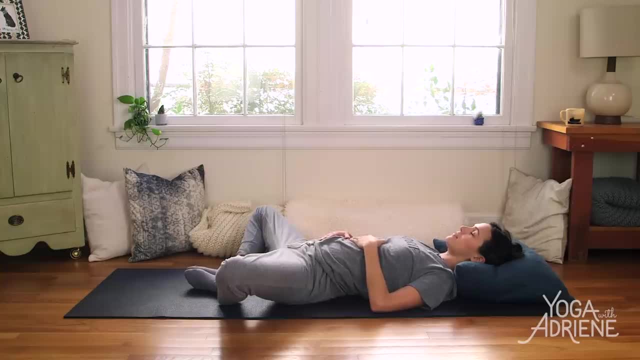 Fill the belly with air. So the hands are gonna rise And then as you exhale they fall nice and slow with control. Inhale belly rises just like a big wave. Maybe there's a small pausing at the top. 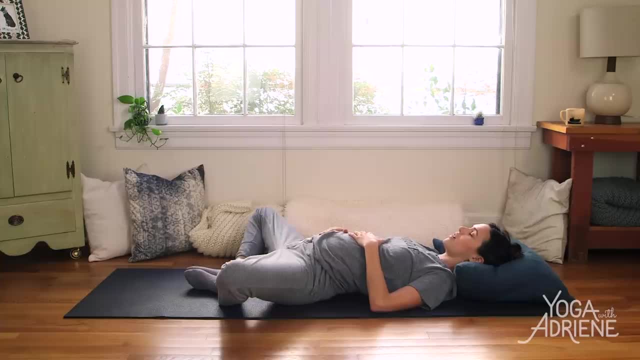 And then exhale. the wave crashes and falls with control. Hands float down, Exhale. Keep this going on your own for just a couple more breaths: Inhaling, belly rises, Exhaling, falling down, Inhale. 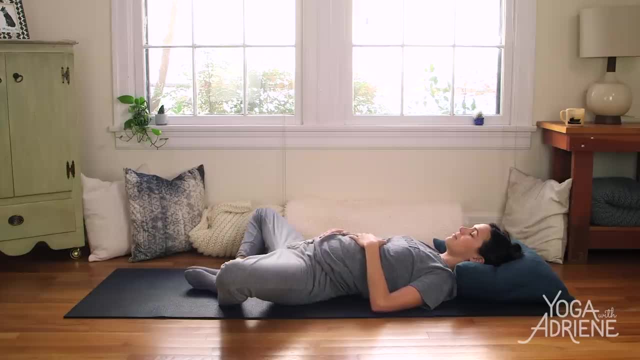 Exhale, Inhale, Exhale, Inhale, Exhale, Exhale. That happens right here. Relax, Relax the jaw here, Surrender, Noticing the sensations in the lower body, The shoulder joints. 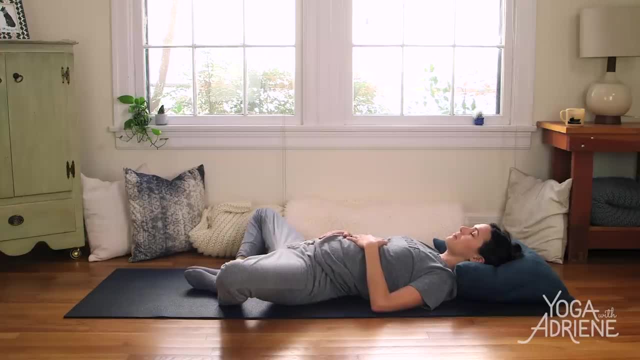 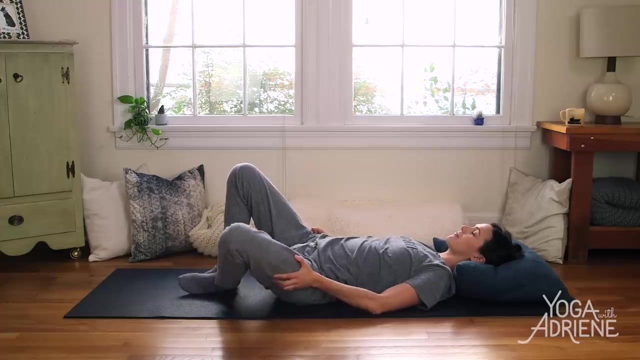 The neck, gracefully slide your fingertips all the way to the outer edges of the legs. You do not have to look at the video here. We're gonna slowly close the legs, one at a time, bringing the knees in, And then I'm gonna lift the knees, give myself a big hug. 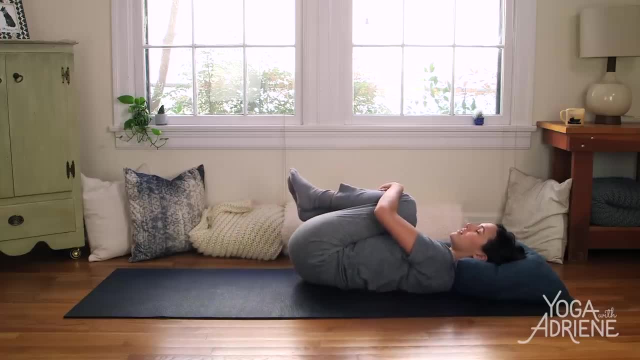 Lower back should feel awesome here. Rock a little side to side, Keep the eyes closed and the breath still going, Maybe draw a couple circles here with the knees, And then I'll slowly release the soles of the feet back to the mat. 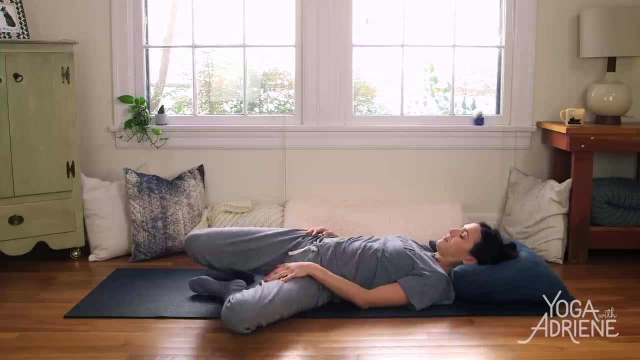 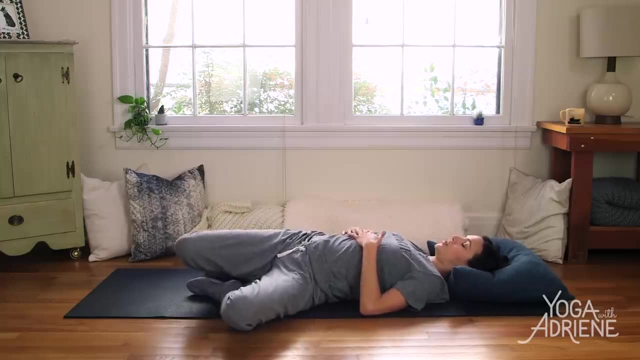 I'm gonna allow the knees to melt over towards the left, Allow your hands to rest gently on the ribcage of the belly here, And what I'm gonna do is just kind of shimmy my shoulders down so that my right knee can really reach. 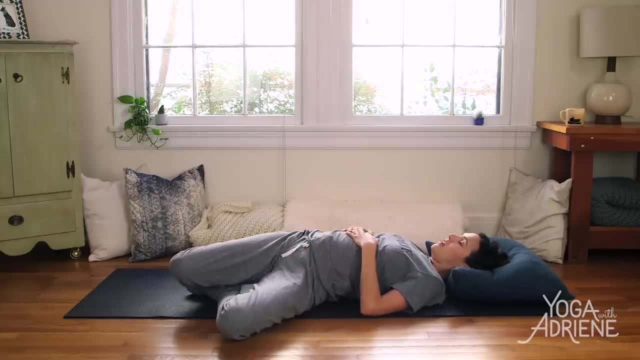 towards the bottom left corner of my mat, Inhale in deeply, Exhale, Release and chill. If you want a little more stretch, you might cross the left, ankle gently over the top of the right, Breathe deep here. 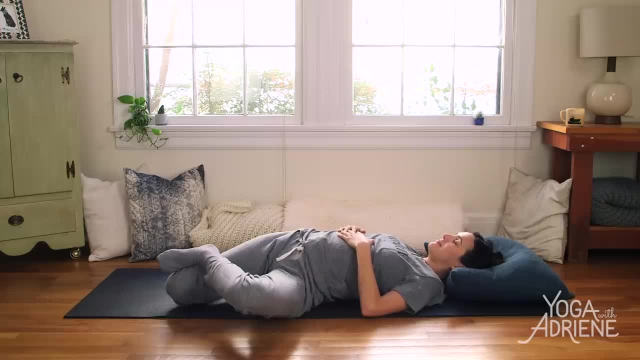 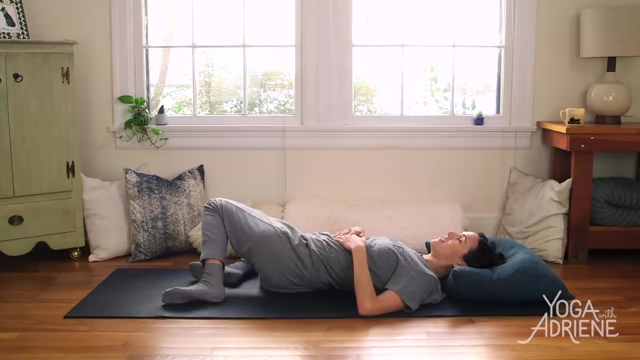 Sink into the earth. Inhale lots of love in, Exhale release, Take it to the other side. So great After a long day, a hard day's work, massaging the booty as you rock over to the right. 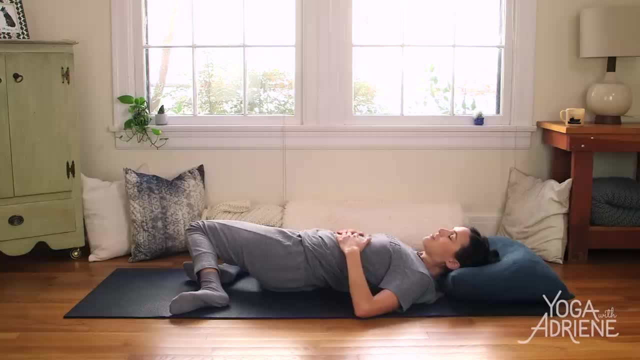 and then the same thing here: drawing the left knee down, resting the weight of the body completely and fully into the earth, Cross the right ankle over the left thigh, if you'd like, and breathe. Hopefully you're starting to feel a little relaxed. 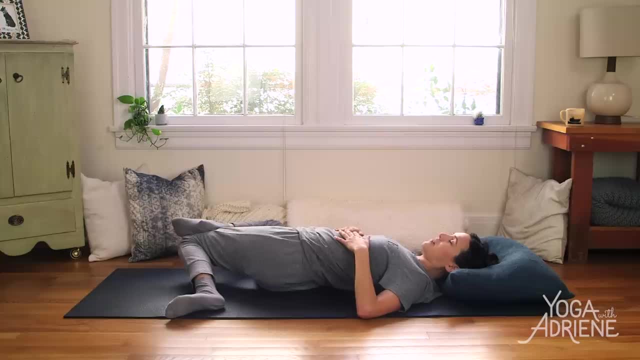 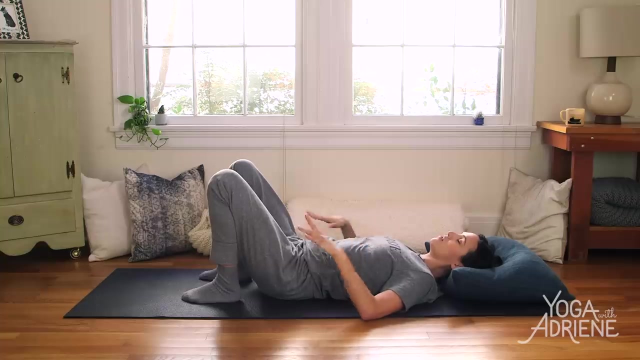 Soften the tongue and the base of the mouth, Begin to let go. Great, we'll slowly rock back to center. Two options here. If you're really sleepy and you feel awesome, move into Shavasana. Otherwise you can take a bridge pose. 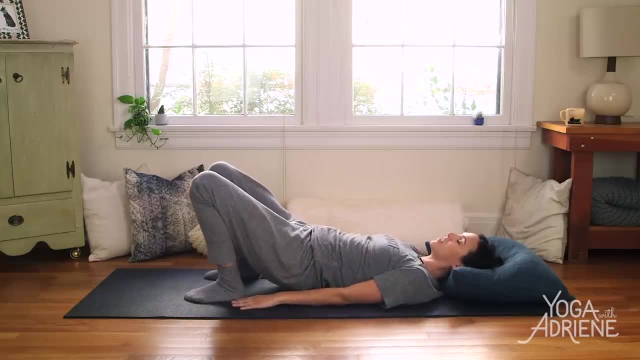 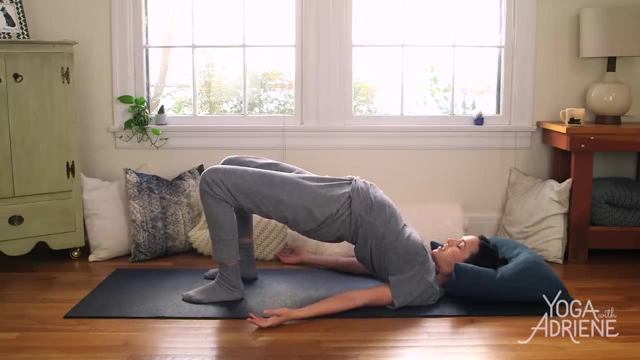 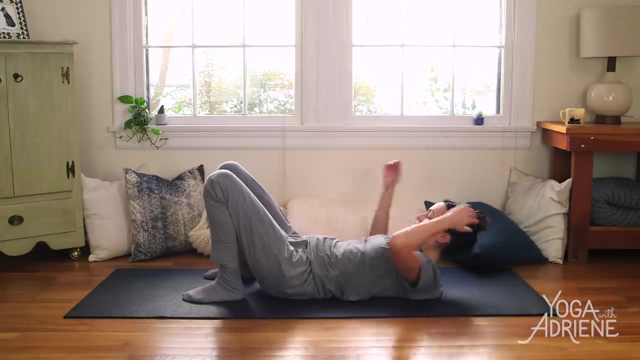 planting the palms And keeping it nice and soft and fluid. As you inhale, lift the hips up, Massaging through the spine, opening up through the palms, And exhale, floating it down. So Shavasana bridge pose or another option. 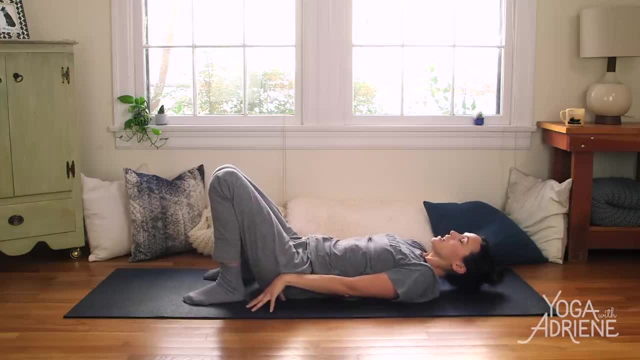 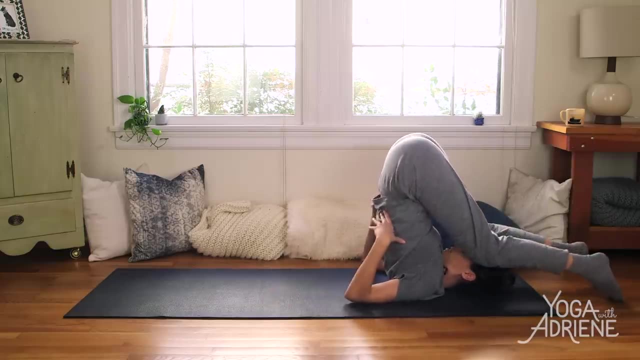 just because I want to take care of all my brothers and sisters out there. all different levels is to crawl the shoulder blades under and come into a little shoulder stand or a plow, So I like to do this. This is really nice. 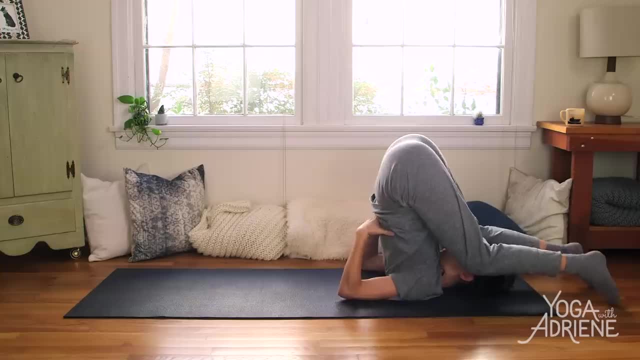 I'm not pushing nice and soft in the feet. Hands come to the lower back body, Knees come to shield the eyes or even the ears, And I just take a breath or two here. So, wherever you are, breathe, Be present with your breath.